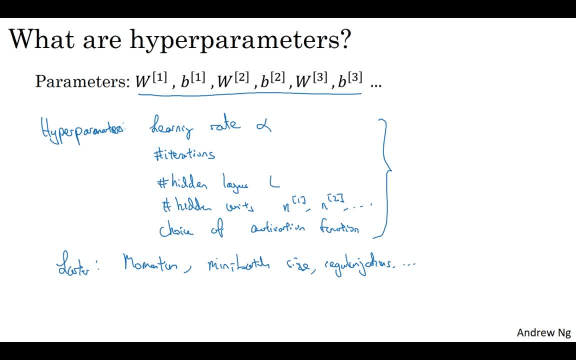 Because deep learning has so many hyperparameters in contrast to earlier areas of machine learning. I'm going to try to be very consistent in calling the learning rate alpha a hyperparameter rather than calling it a parameter, I think in earlier areas of machine learning. 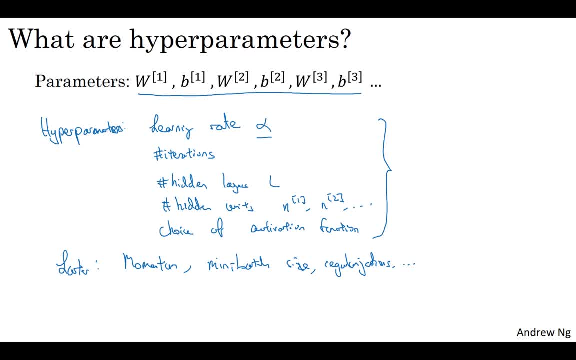 when we didn't have so many hyperparameters, most of us used to be a bit sloppier and just call alpha a parameter. And technically alpha is a parameter, but it is a parameter that determines the real parameters. So I try to be consistent in calling these things like alpha. 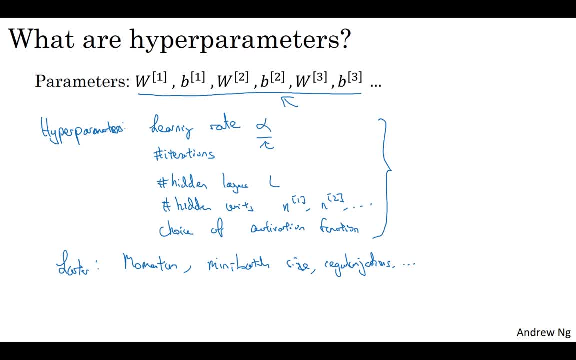 the number of iterations and so on, hyperparameters. So when you're training a DeepNet for your own application, you find that there may be a lot of possible settings for the hyperparameters that you need to just try out. So applied deep learning today is a very empirical process. 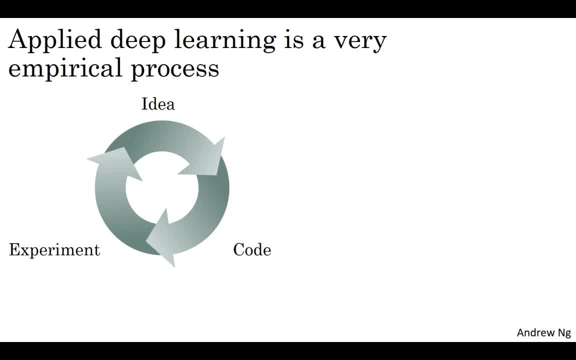 where often you might have an idea. For example, you might have an idea for the best value for the learning rate. You might say, well, maybe alpha equals 0.01, I want to try that. Then you implement it, try it out and then see how that works. 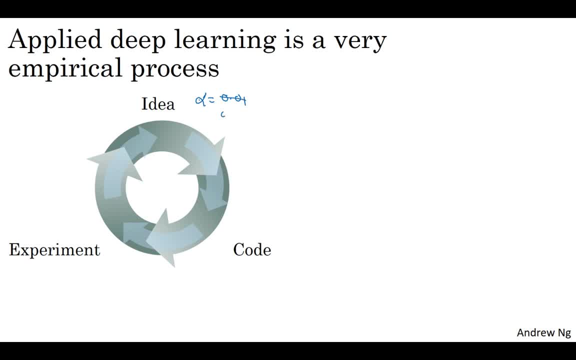 And then, based on that outcome, you might say: you know what? I've changed my mind. I want to increase the learning rate to 0.05.. And so, if you're not sure what's the best value for the learning rate to use, 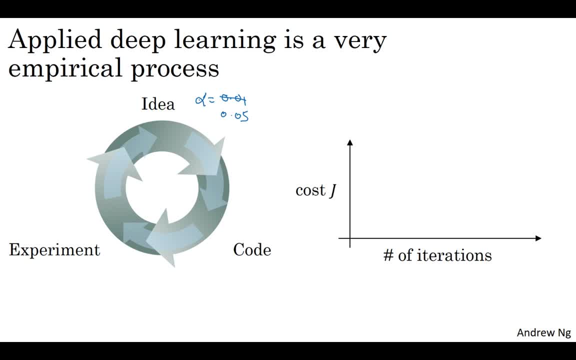 you might try one value of the learning rate alpha and see the cost function j go down like this. Then you might try a larger value for the learning rate alpha and see the cost function blow up and diverge. Then you might try another version. 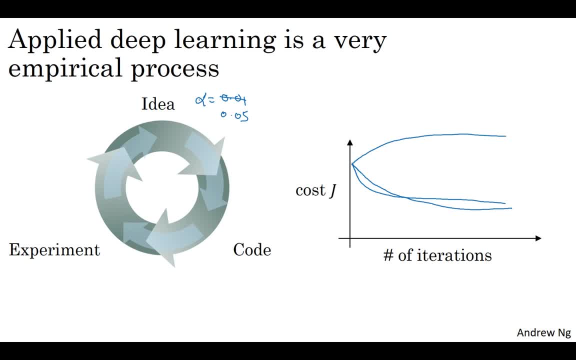 and see it go down really fast but converts to a higher value. You might try another version and see the cost function. j do that. Then, after trying to set the values, you might say, okay, it looks like this, the value of alpha. 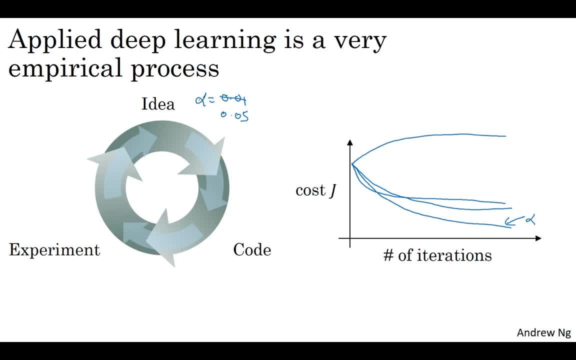 gives me a pretty fast learning and allows me to converge to a lower cost function j. So I'm going to use this value of alpha. You saw in the previous slide that there are a lot of different hyperparameters And it turns out that when you're starting on a new application, 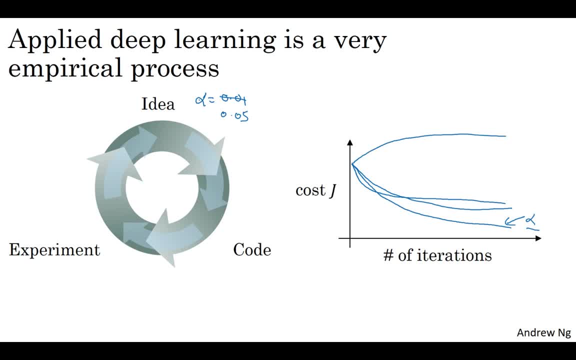 I actually find it very difficult to know in advance exactly what's the best value of the hyperparameters. So what often happen is you just have to try out many different values and go around the cycle. You try out some value, maybe you try five hidden layers with this many number of hidden units, 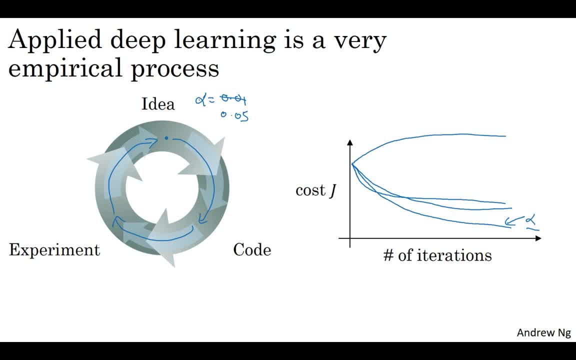 implement that, see if it works and then iterate. So the title of the slide is that Applied Deep Learning is a very empirical process. An empirical process is maybe a fancy way of saying you just have to try out a lot of things and see what works. 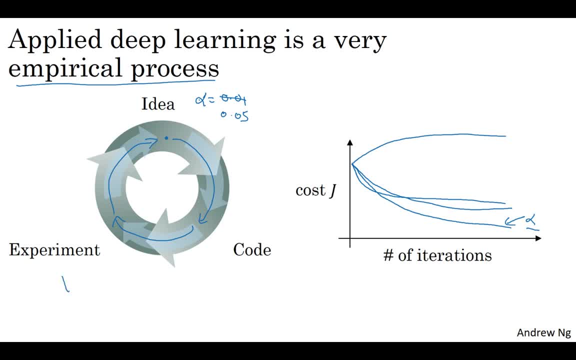 Another effect I've seen is that deep learning today is applied to so many problems, ranging from computer vision to speech recognition, to natural language processing, to a lot of structured data Applications such as maybe online advertising or web search or product recommendations and so on. 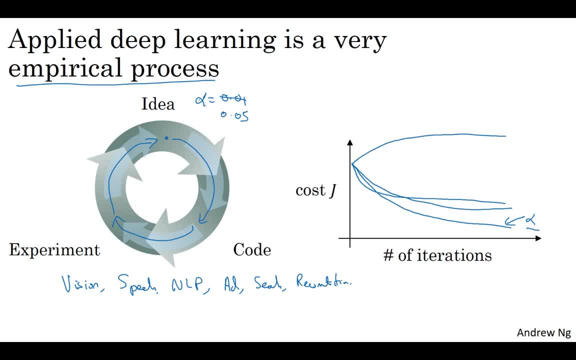 And what I've seen is that first I've seen researchers from one discipline. any one of these try to go to a different one, and sometimes the intuitions about hyperparameters carries over, and sometimes it doesn't. So I often advise people. 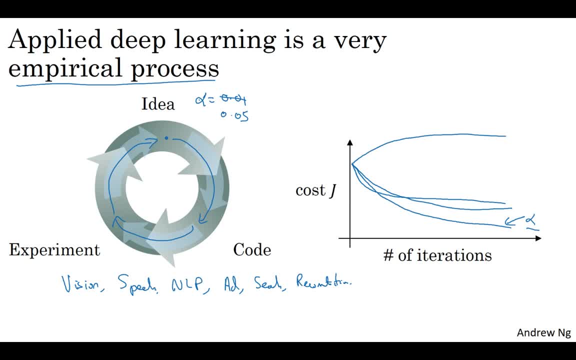 especially when starting on a new problem, to just try out a range of values and see what works. And in the next course we'll see a systematic way, We'll see some systematic ways for trying out a range of values. And second, even if you're working on one application for a long time, 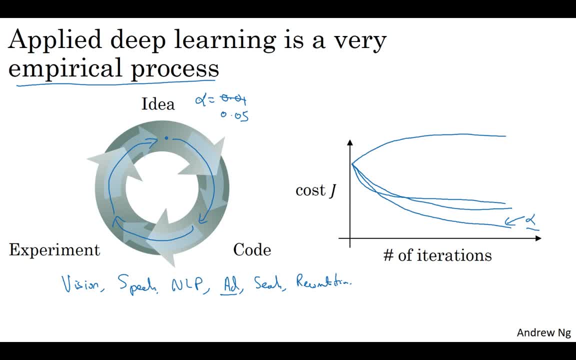 maybe you're working on online advertising. as you make progress on the problem, it's quite possible that the best value for the learning rate, the number of fitting units and so on might change. So even if you've tuned your system to the best value of hyperparameters today, 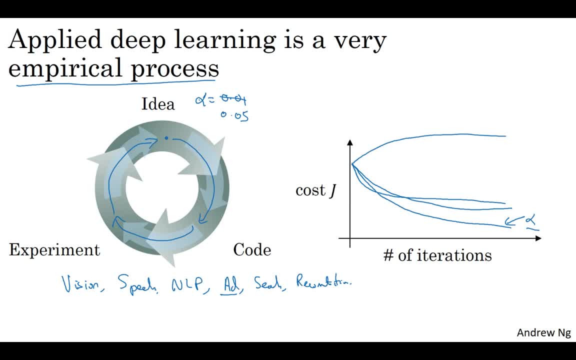 it's possible you find that the best value might change a year from now, Maybe because the compute infrastructure- be it you know CPUs, or the type of GPU you're running on, or something- has changed. But so maybe one rule of thumb is: you know every now and then. 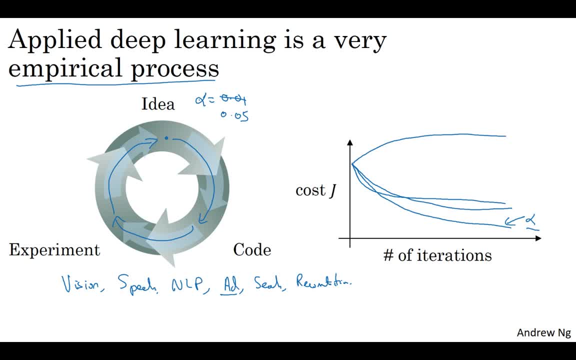 maybe every few months if you're working on a problem for an extended period of time, for many years, just try a few values for the hyperparameters and double check if there's a better value for the hyperparameters, And as you do so, you slowly gain intuition as well about 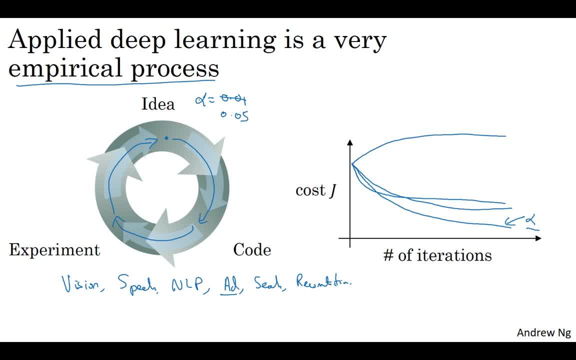 the hyperparameters that work best for your problem, And I know that this might seem like an unsatisfying part of this, but, you know, I think that this is a good thing. I think that this is a good thing, And I know that this might seem like an unsatisfying part of the problem. 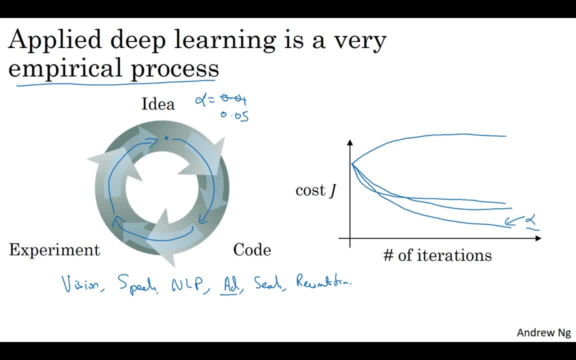 And I know that this might seem like an unsatisfying part of the problem, And I know that this might seem like an unsatisfying part of deep learning- that you just have to try a lot of values for these hyperparameters, But maybe this is one area where deep learning research is still advancing.